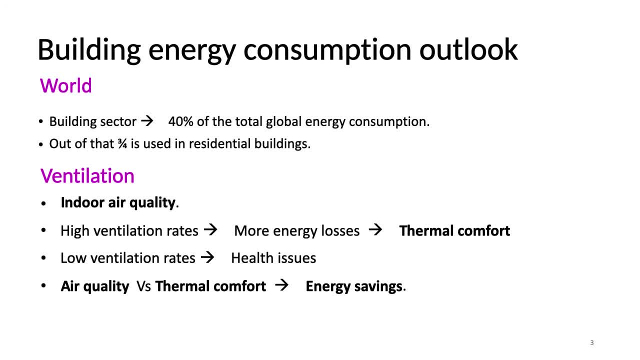 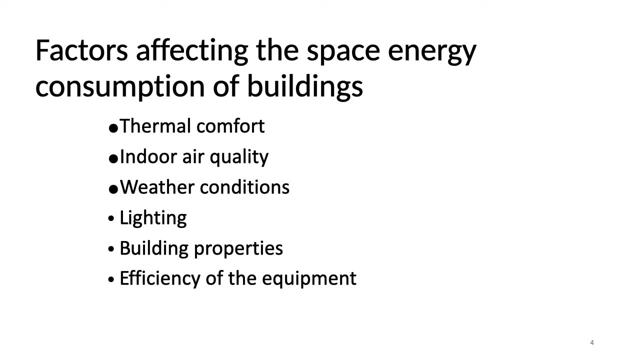 low rates can give rise to health issues. Therefore, there is a compromise between the air quality and the thermal comfort when it comes to energy savings in buildings. There are various factors that affect the energy consumption of buildings, such as thermal comfort, indoor air quality. 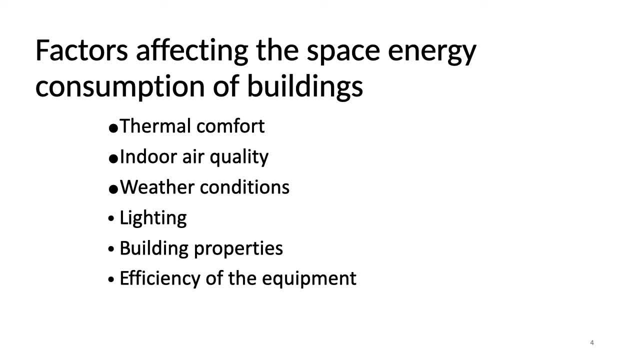 weather conditions, lighting, building properties and efficiency of the equipment. To obtain optimal energy performance, it is necessary to integrate the effects from each and every fact mentioned here. It can be carried out via a precisely selected building control system to maintain the thermal comfort of occupants and to achieve good energy efficiency For good building. 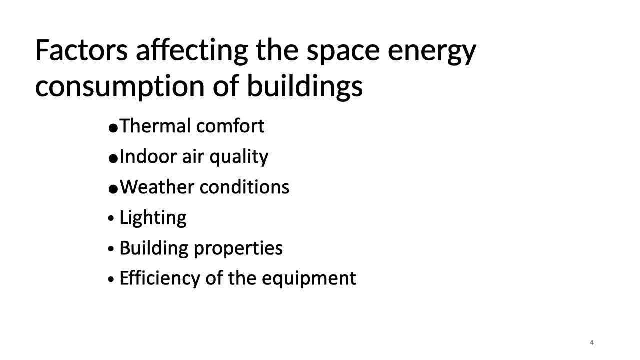 control systems. it is necessary to have a good model that mimics the properties of the building. So let's move on to see how a mathematical model of a heater single zone building is developed for prediction of temperature. Here is the building system we are interested in modeling: The whole building is. 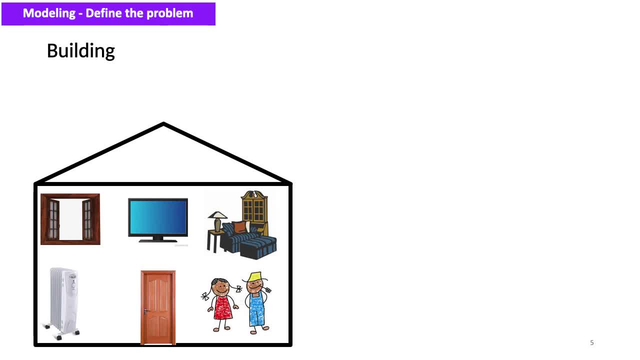 considered as one unit and we are going to address the heat losses from walls, roof, windows and doors to the outside, heat losses from ground floor to the earth, ventilation, heat losses, thermal mass of the building and temperature, The heat generation from heaters, electrical equipment and people. These are the 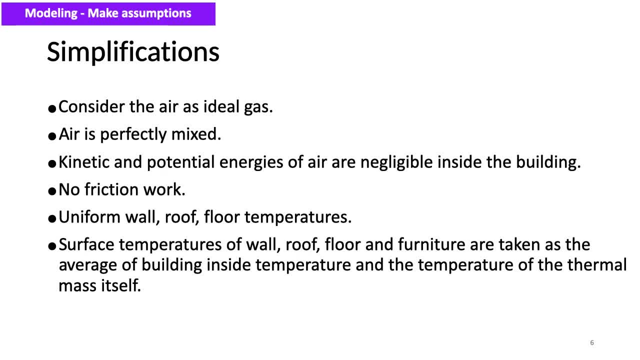 simplifications or assumptions we used in this modeling task. Consider the air as an ideal gas and perfectly mixed. Kinetic and potential energies of air are negligible inside the building. No friction work, an uniform wall roof flow temperatures, Surface temperatures of walls, roof, floor and furniture are. 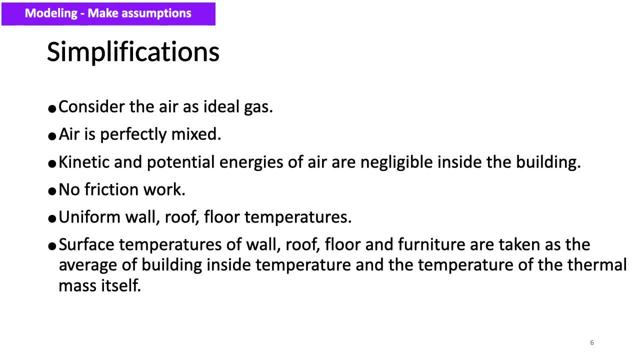 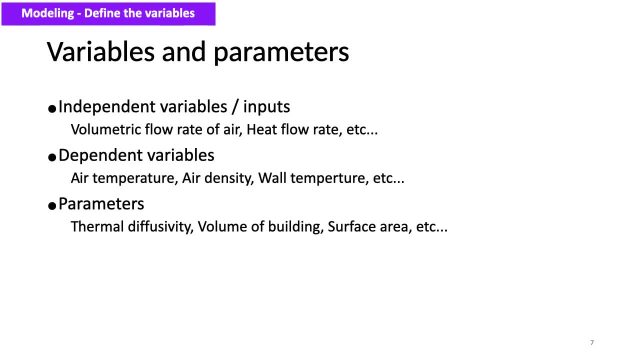 taken as the average of the building inside temperature and the temperature of the thermal mass itself. In the model you can find independent variables or inputs, dependent variables and parameters. The two dependent variables we are interested in in this model are air density and air temperature. Inputs to the model are volumetric flow. 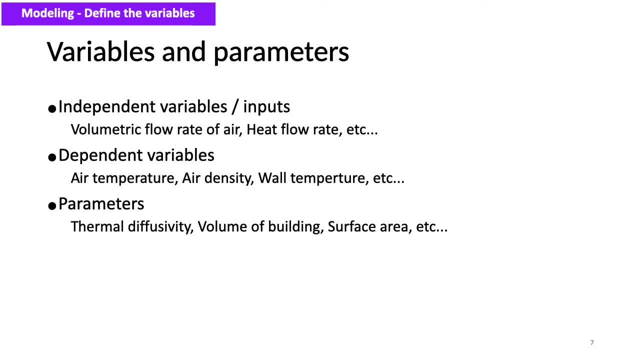 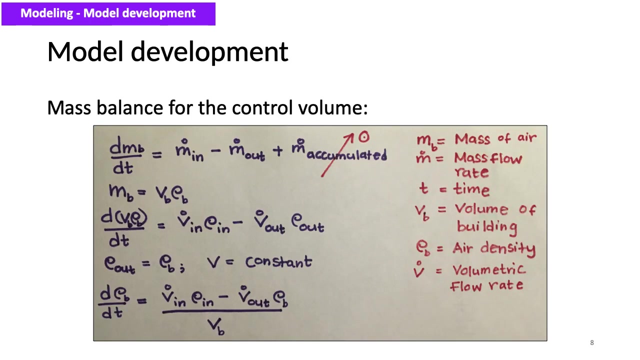 rate of air, heat flow rate, solar irradiation and so on. There are many parameters in the model, such as thermal diffusivity, volume of building surface area, etc. We will talk further about different variables at the development stage. So now we have come to the modeling part of this video. A continuous 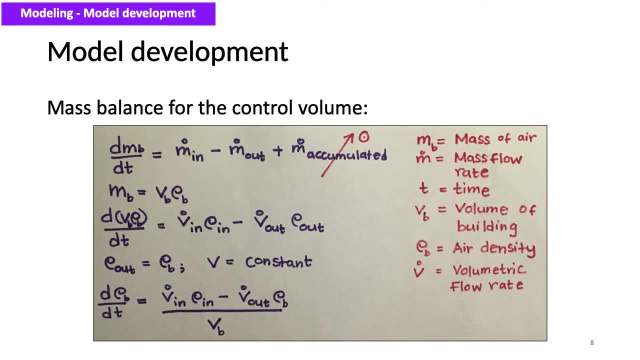 time dynamic heating model is developed based on the first principles for the mentioned building unit and it is considered as a control volume. The model is expressed in terms of state space variables and a lumped parameter approach has been used for estimations. As we have seen in the previous video, the dynamic heating model is used for 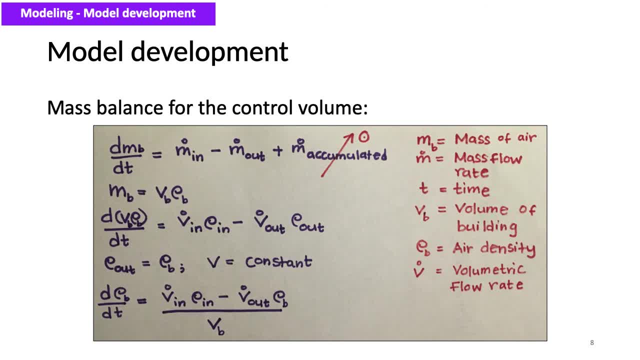 ventilation plays a leading role in the convective mode of heat transfer in buildings. The application of mass balance to the air flow is therefore vital in the modeling of ventilated spaces. The representative mass balance equation for a single zone building unit of volume, Vb under perfectly mixed 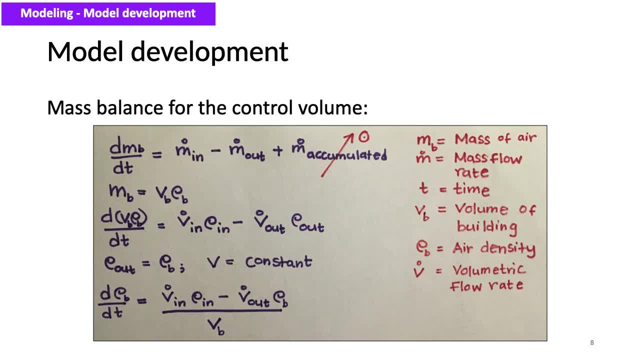 conditions can be written as given. in this equation, Air is admitted as an ideal gas, having both dry air and water vapor. Here the mass accumulation term goes to zero because there is no mass accumulation inside the building and the mass of the air can be represented as a. 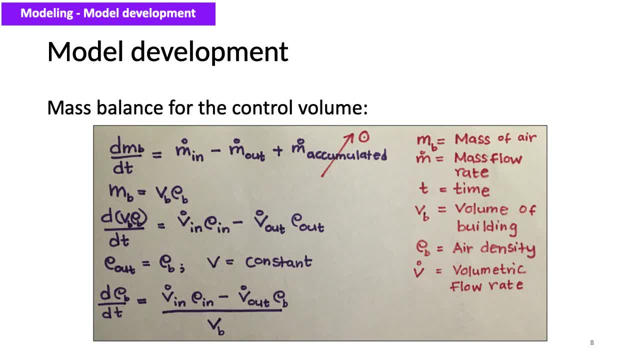 product of volume times the density. The density of air flowing out of the building is equal to the density of air inside the building. because we assume that air is perfectly mixed, The volume of the building is a constant and hence we can take that term out and can represent 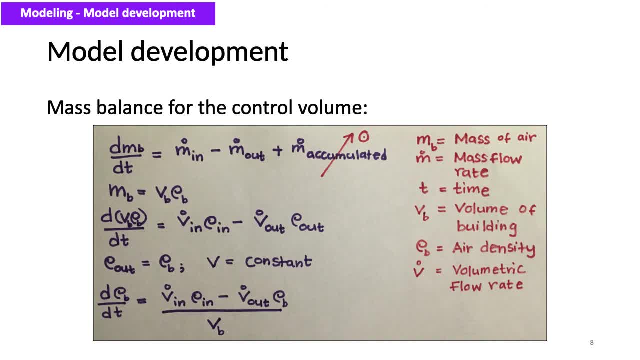 the equation in this form. These are the terms we used in this equation: development: Mb represents the mass of air inside the building. Mdot is the mass flow rate of air. Simple t is the time. Vb is the volume of the building. 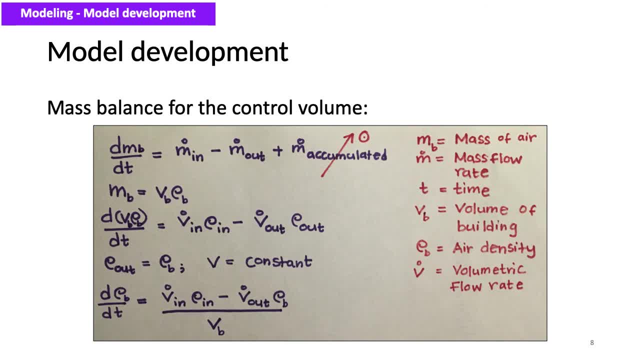 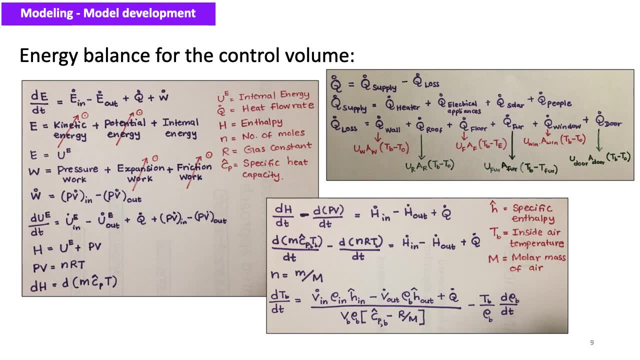 Rb is the air density inside the building, Vdot is the volumetric flow rate of air. The energy balance equation for the building unit is developed using the general energy balance considering a control volume. Eb is the total energy of the control volume, which consists of kinetic potential and internal energies. 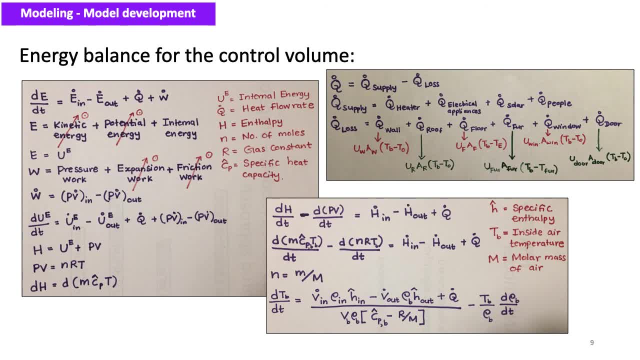 Air flow velocity. the single zone building unit is small, hence kinetic energy is not taken into consideration. the potential energy of the system is also of minor importance, so only the internal energy term is taken into account, and W is the combination of which pressure work, expansion work and friction work as the 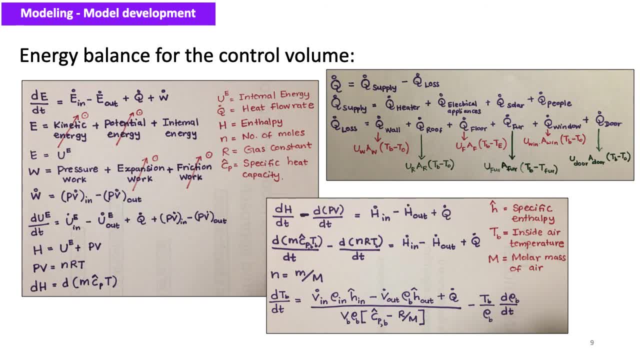 volume of the room is fixed, expansion work is zero. friction work is also close to zero because AI is the fluid of interest. pressure work is the only term that is relevant in the energy transfer by work in this model and considering three relations: H equals U plus PV, PV equals nRT and dH equals dMcp. 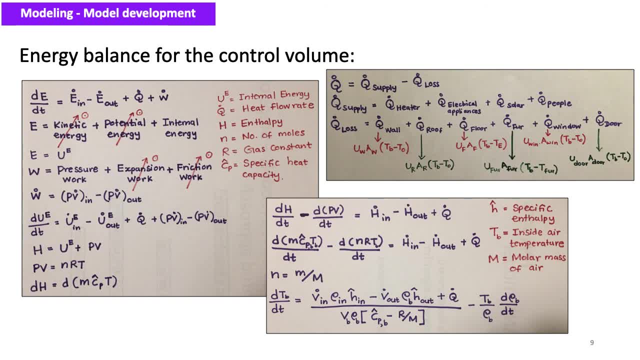 T, we can derive the energy balance equation into this final form and Q dot is the total heat flow rate from sources other than ventilation, and it is equal to Q dot supply minus Q dot loss. Q dot supply is the energy supplied by heaters, electrical equipments, solar irradiation and. 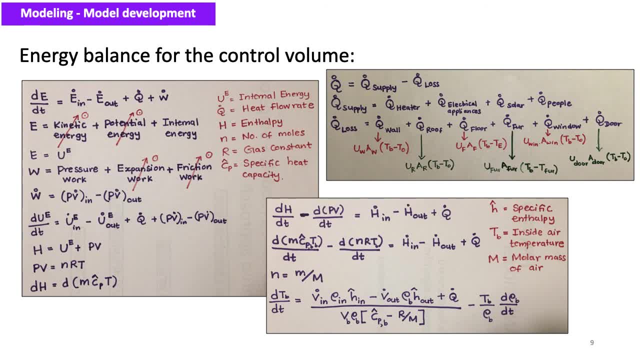 because of people, and the terms of energy losses are energy losses through the walls, through the roof, through the flow, through furniture, and through the windows and through the doors. the heat losses can be represented as u, a, delta, t, where U is the overall heat transfer coefficient, a is the surface area of heat. 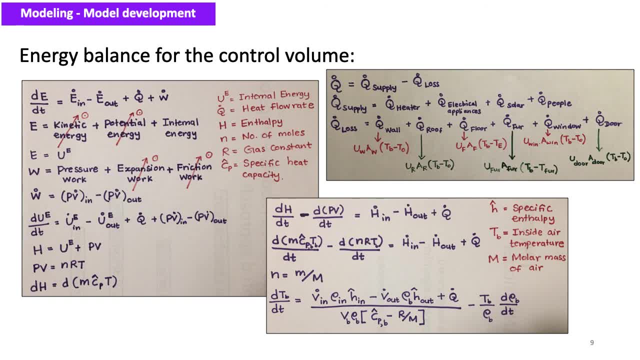 transfer, and there the T is the temperature difference. and these are the terms used in this equation: U, E is the internal energy, Q, dot is the heat flow rate, H is the enthalpy, N is the number of moles of air, R is the gas constant and C hat P is the specific heat. 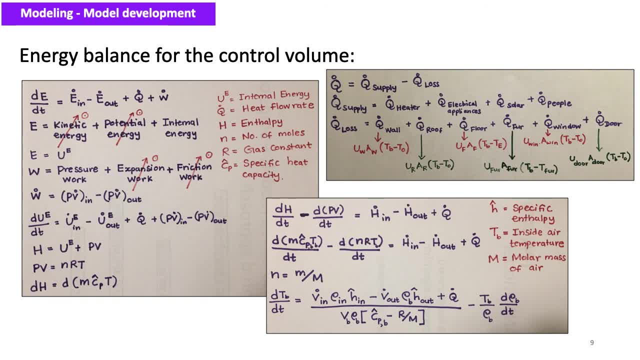 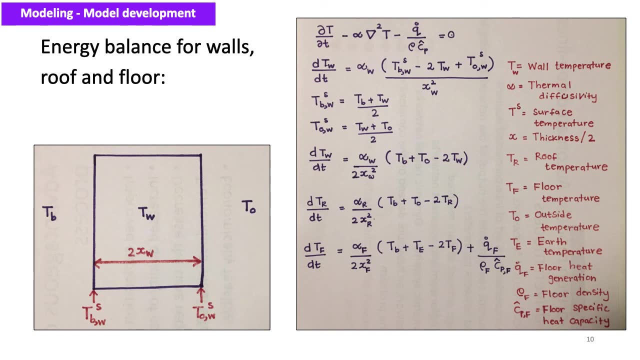 capacity. H hat is the specific enthalpy, T B is the inside air temperature. capital M is the molar mass of air. the building envelope is fabricated using layers of dissimilar materials. the volume in between the innermost and outermost wooden boards is loaded with insulation materials. 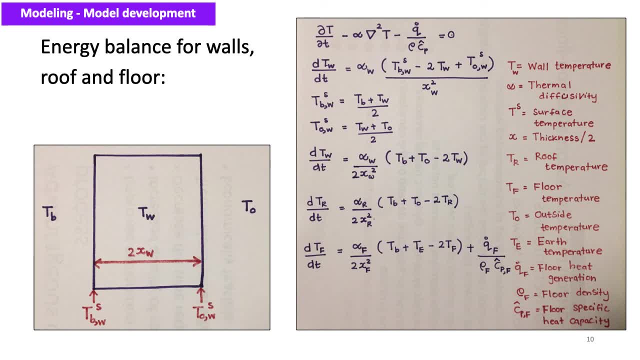 and vapor barriers to overcome the heat losses. Transient heat equation is used to derive one-dimensional heat transfer equations for different layers of the building envelope. To simplify the problem, transient heat equation is transformed to ordinary differential equation using the finite difference method and it is assumed that the temperature throughout. 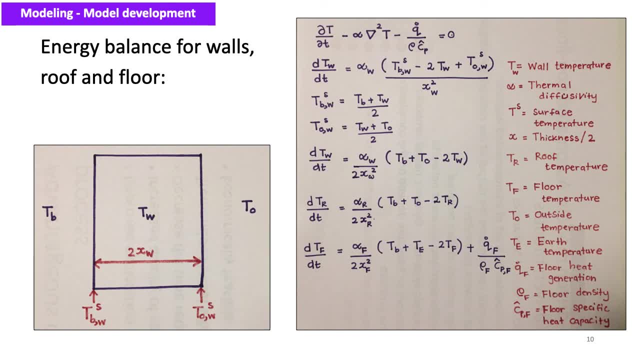 the envelope is uniform for simplifications. Further, the surface temperatures are approximated as the mean temperature of the neighboring layers. The same principle has been applied for wall, roof and flow temperature models, except that flow is having an internal heat generation term, such as flow heaters. 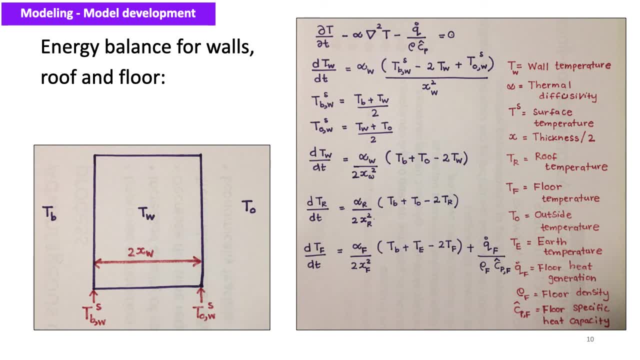 And because of the simplifications I used in estimating the surface temperatures of the building envelope, I did not use the complex boundary condition equations in this model. In the next video, I will show you how to use the complex boundary condition equations in this model. 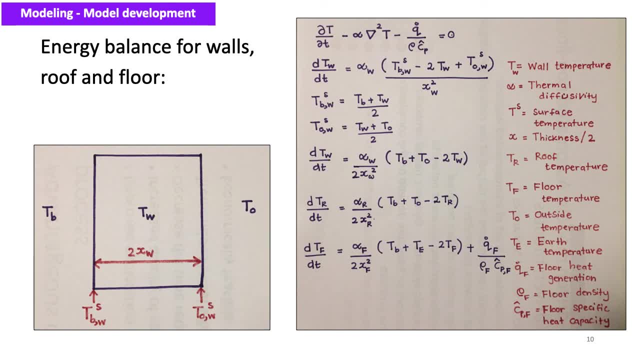 But if you want to estimate the surface temperatures more accurately, then you can write an equation relating the conduction and convection heat transfer at the surface of this property. The symbols used in this equation are: T. w is wall temperature, alpha is the thermal diffusivity. T superscript x is the thermal. 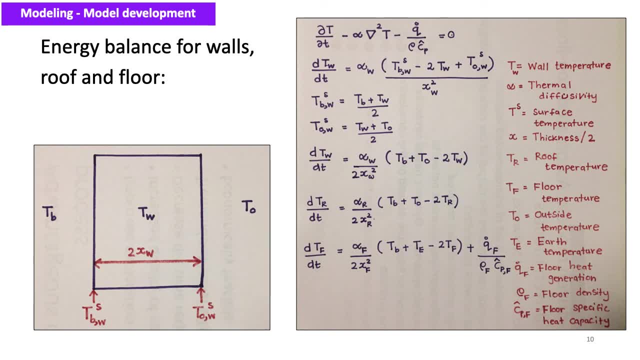 diffusivity. T. w is wall temperature. alpha is the thermal diffusivity T superscript x is the thermal diffusivity. T s is the surface temperature. simple x is the thickness divided by 2, T r is the roof. 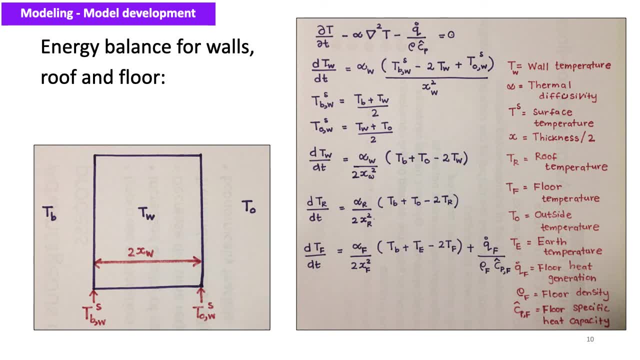 temperature. T f is the floor temperature, T o is the outside temperature, T e is the earth temperature, otherwise ground temperature. Q dot f is the floor heat generation, Rho f is floor density, CPF, hat is the flow specific heat capacity. 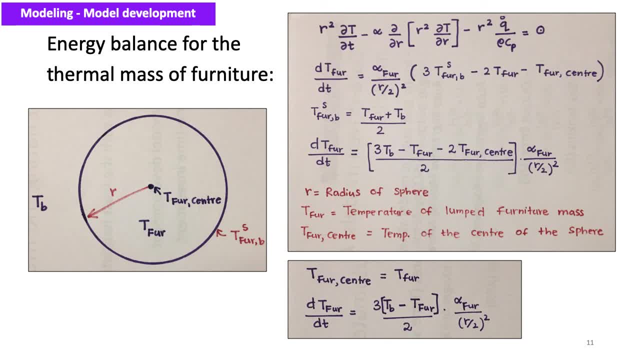 The modeling of household furniture, including internal walls, is important when modeling the buildings. They act as either heat sink or heat source, depending on the temperature difference between themselves and the surrounding air. The availability of furniture prolongs the heating and cooling times of buildings. To simplify the modeling approach of furniture, it is defined: 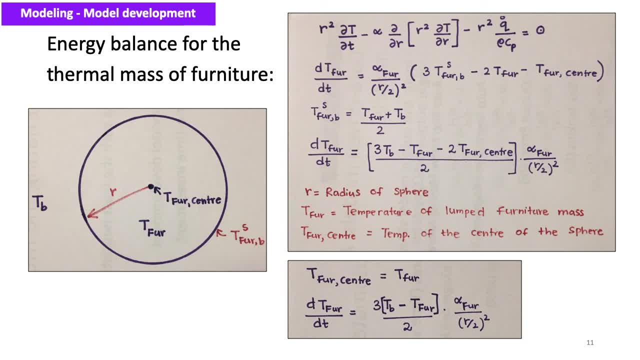 as a spherical object with the equal mass and equivalent average thermal diffusivity. The heat equation in spherical coordinates is given by this equation and we can use finite difference method to discretize this equation. After discretization, use the average temperature of furniture and inside air as the surface temperature of the furniture and use the center. 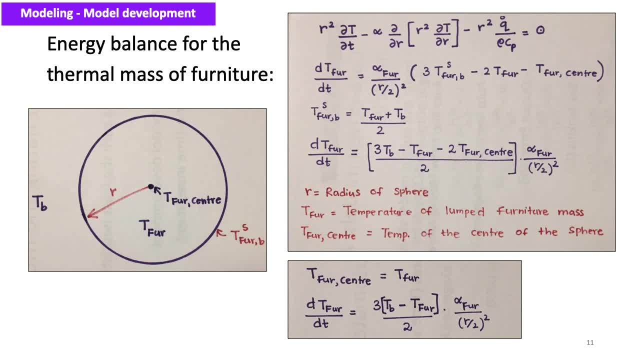 temperature of furniture as the furniture temperature. Then you can come up with this final simplified equation for the energy balance for furniture. Simple r represents the radius of sphere, Tfer is the temperature of lumped furniture mass and Tfer center is the temperature of the. 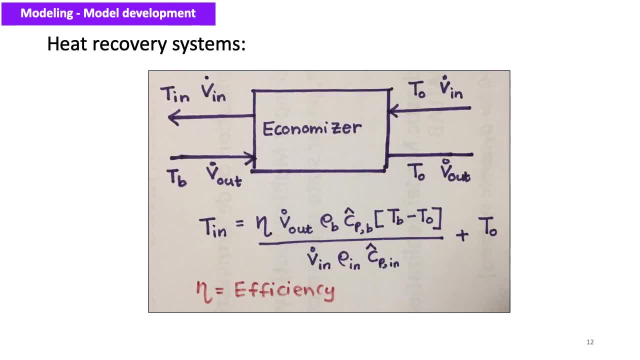 center of the sphere. Usually, the ventilation system of a building is integrated with an economizer or heat recovery system. In this system, the incoming air will be heated by the warm air flowing outside of the building. The temperature of the incoming air flow can be assessed using an. 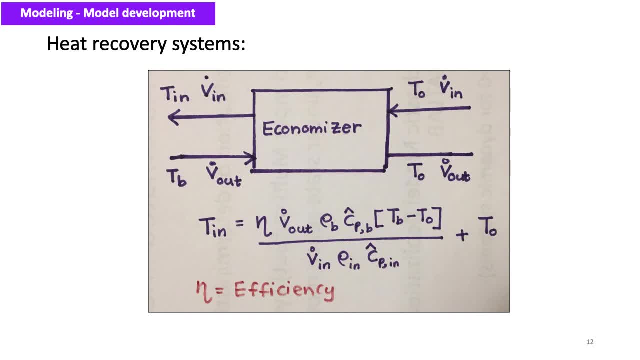 energy efficiency, eta, and with the assumption of equal densities and specific heat, If the energy is not equal to the heat capacity in the two counter current air flow streams Having this installation, the thermal properties of the inlet air should be estimated by use of Tin, which is the 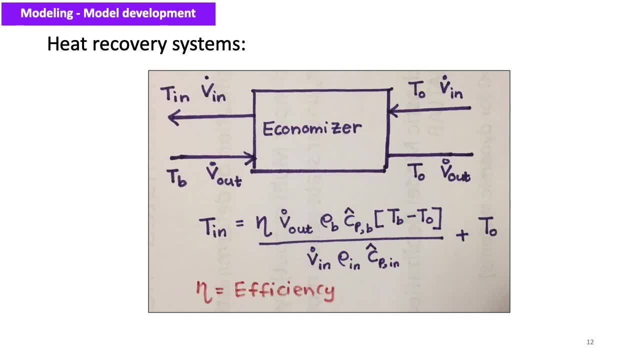 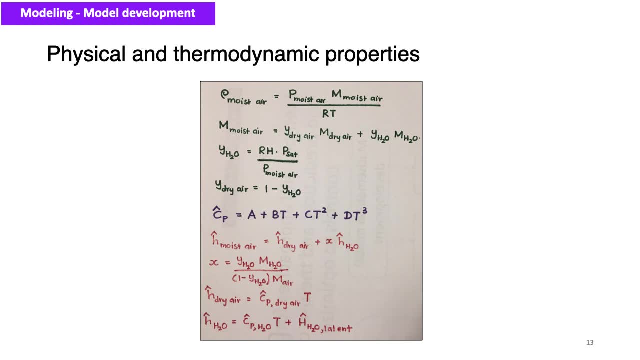 incoming air flow temperature rather than To, which is the outside temperature of the building. The important physical and thermodynamic properties that are useful in further analysis of this model is given here. The density of moist air can be approximated using the ideal gas equation, and it is equal to pressure of moist air times. molar mass of moist air divided by R. 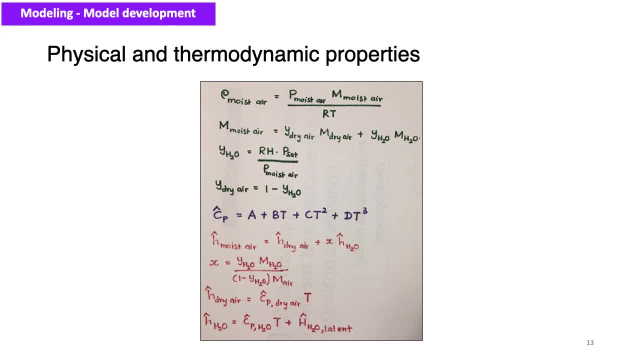 into T. R is the gas constant and T is the temperature of moist air. Molar mass of moist air is equal to molar fraction of dry air times molar mass of dry air plus molar fraction of water times molar mass of water. The 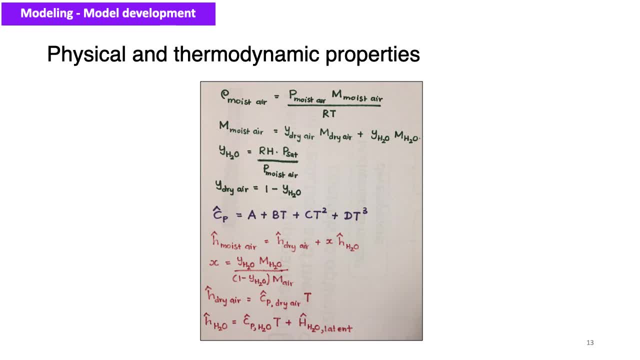 molar fraction of water can be calculated using relative humidity times. saturation pressure divided by the pressure of moist air and the specific heat capacities can be calculated using the equation: Cp equal to T. R was a plus bt plus ct, squared plus dt to the power 3.. So these constants, a, b, c, d, can 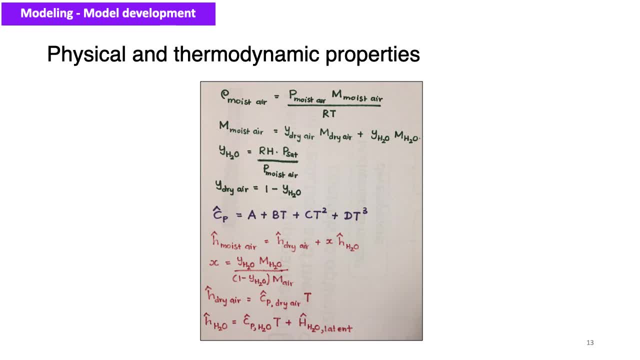 be found in thermodynamic property tables for moist air. The specific enthalpy of moist air is equal to specific enthalpy of dry air, plus x times specific enthalpy of water. x is the ratio between molar fraction of water times molar mass of water divided by molar. 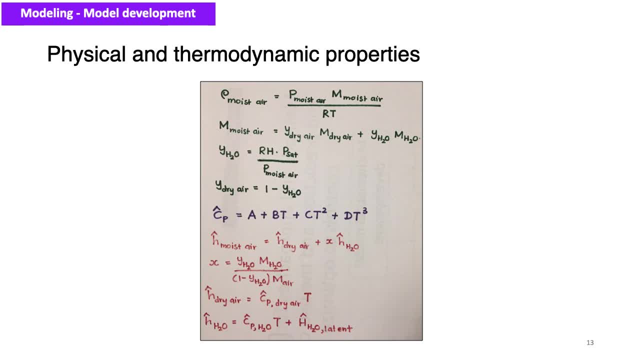 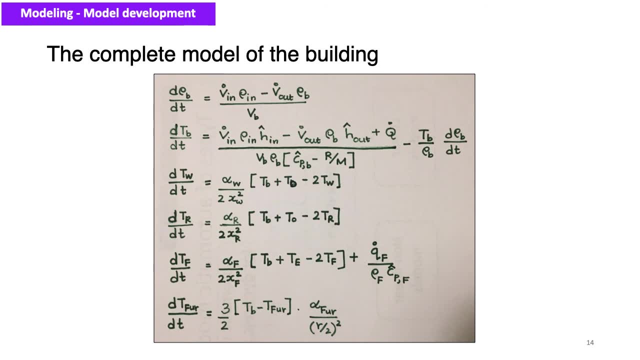 fraction of dry air times. molar mass of dry air. This is the complete model of the building and it is in the state space form. There are six dependent variables, and they are: density of air, temperature of air temperature of the wall, temperature of the roof, temperature of the floor and temperature of the furniture.